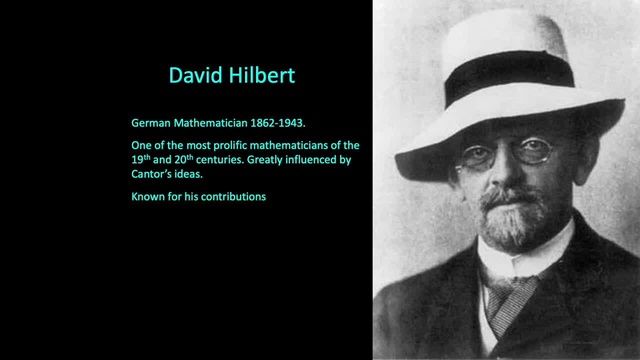 greatly influenced by Cantor's ideas. Hilbert's known for his contributions to various areas, including, but not limited to, commutative algebra, mathematical physics, invariant theory and and the Theory of Mathematical Proofs. He's most famous for his presentation in the year 1900. 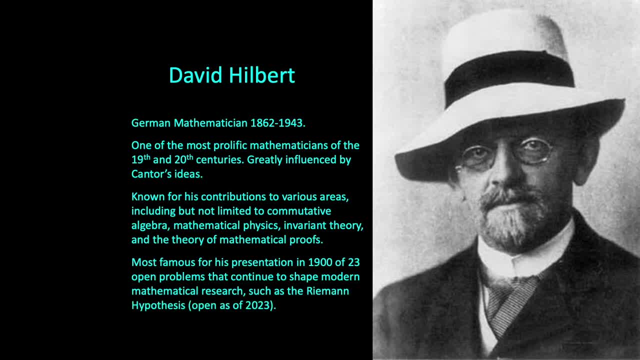 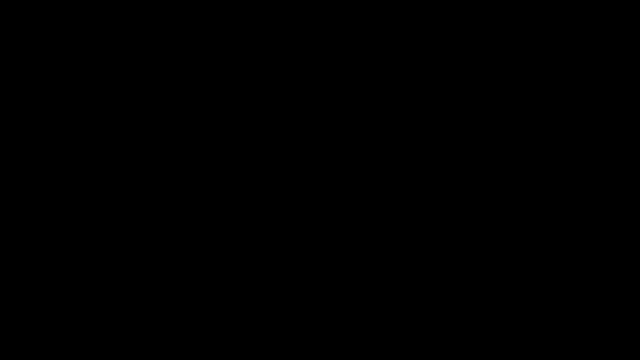 of 23 open problems that continue to shape modern mathematical research, such as the Riemann Hypothesis, which is still open as of 2023.. And Hilbert had 77 doctoral students, which leads us to the most important person in the story of the axiom of choice. 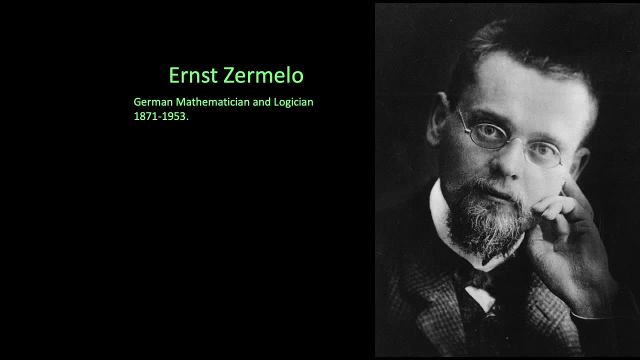 Ernst Zermelo. He was a German mathematician and logician who lived from 1871 to 1953.. He further developed the theory of transfinite cardinals introduced by Cantor. He developed axioms for set theory, just as Euclid did for axioms of geometry. 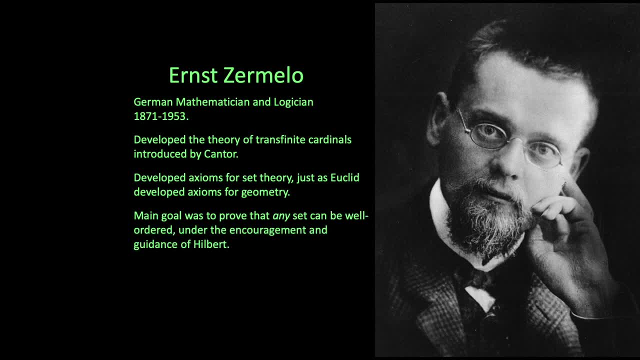 Zermelo's main goal was to prove that any set can be well-ordered, under the encouragement of Hilbert And he introduced the axiom of choice in 1904 as a tool to prove this generalized well-ordering theorem. Now let's look at a more precise statement of the axiom of choice. 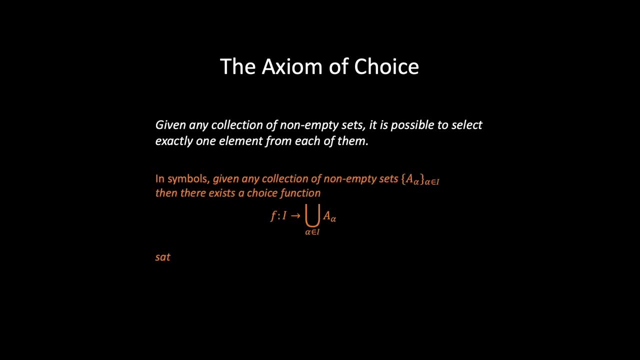 In symbols, given any collection of non-empty sets, A sub alpha. here alpha is an index from some set, I. then there exists a choice function, F from I to the union of all the A's, Such that F of alpha is an element of A sub alpha for each index alpha. 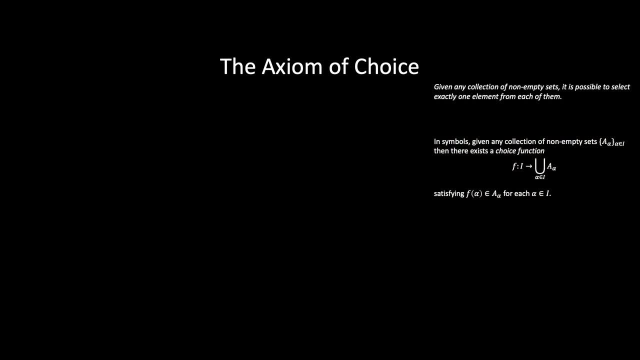 In other words F chooses a specific element from each of the sets A sub alpha. Let's do some examples. Say I is the set whose cardinality equals the number of pairs of shoes in the world- Maybe that's infinite. Then a particular pair of shoes can be denoted by the set A alpha. 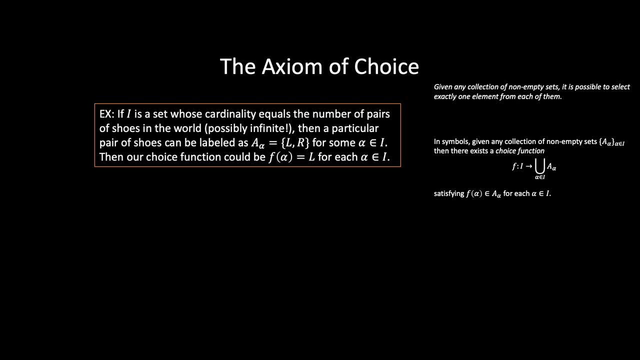 and its elements are L and R for left and right shoe, and our choice function could just be picking the left shoe every time. Now let's do an example where I is the set whose cardinality is the number of pairs of shoes. Again, maybe there are infinitely many socks. 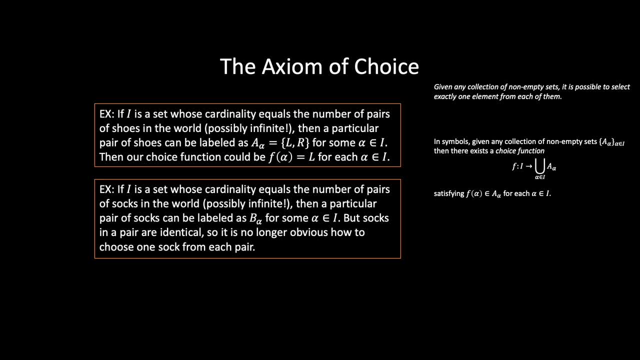 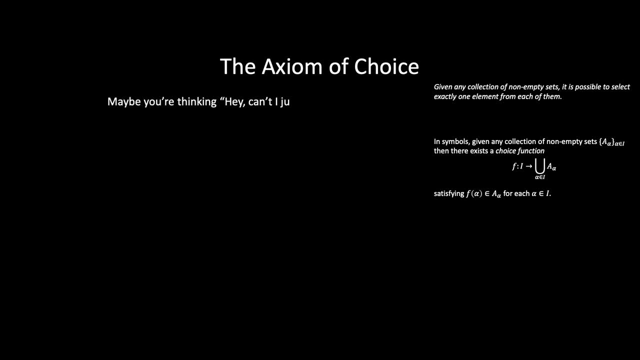 And a particular pair of socks can be labeled as a set B alpha, But socks in a pair are identical, so it's no longer obvious how to choose one sock from each pair. Or maybe you're thinking, hey, can I just use my left hand to pick a sock from each pair. 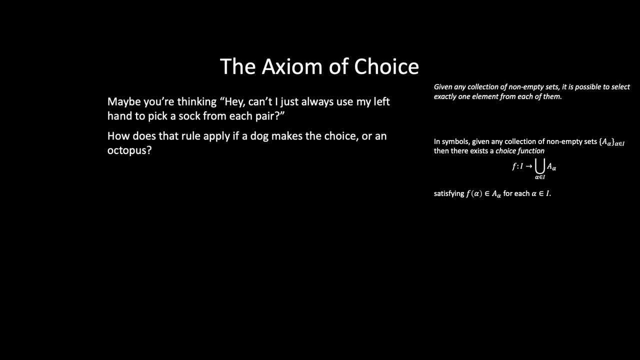 Well, how does that rule apply if a dog makes the choice, or maybe even an octopus? What's their left hand? The point is that the choice function needs to be independent of the entity that makes the choice. The point is that the choice function needs to be independent of the entity that makes the choice. 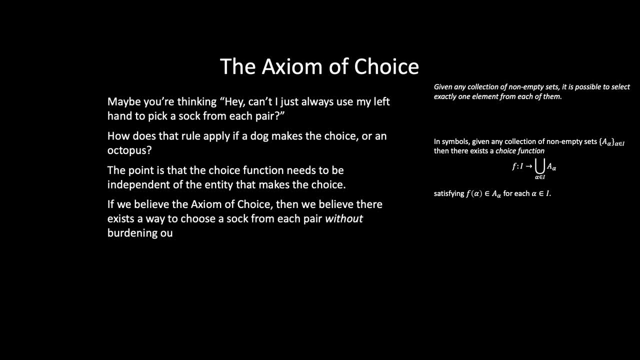 So that would be the idea for today. Okay, believe the axiom of choice, then we believe there exists a way to choose a sock from each pair without burdening ourselves with describing how to do so. This turns out to be a useful additional hypothesis for proving various results in mathematics. Some mathematicians 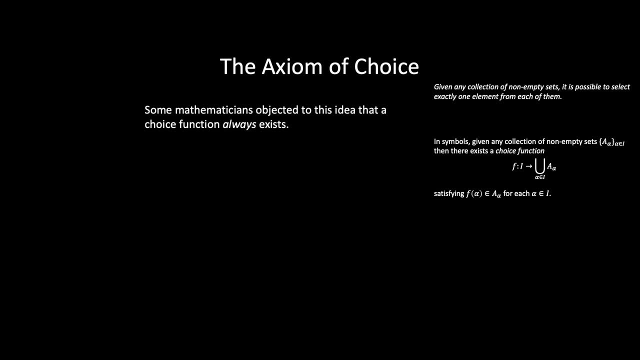 objected to this idea that a choice function always exists. What was particularly unnerving was that the axiom of choice is non-constructive. So, for example, when an uncountable number of choices must be made, the axiom of choice asserts that it's possible to do so without 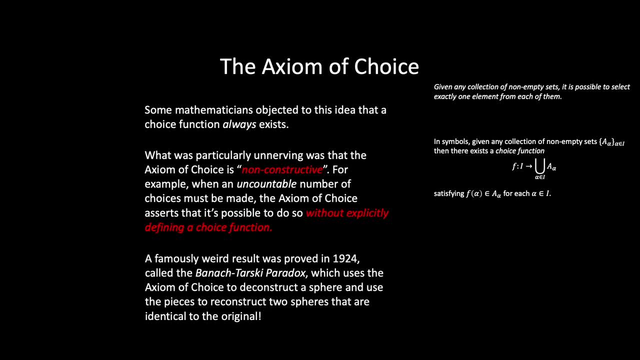 explicitly defining a choice function. A famously weird result proved in 1924, called the Bonn-Oktarski paradox. It uses the axiom of choice to deconstruct a sphere and uses the pieces to reconstruct two spheres that are identical to the original. So on the one. 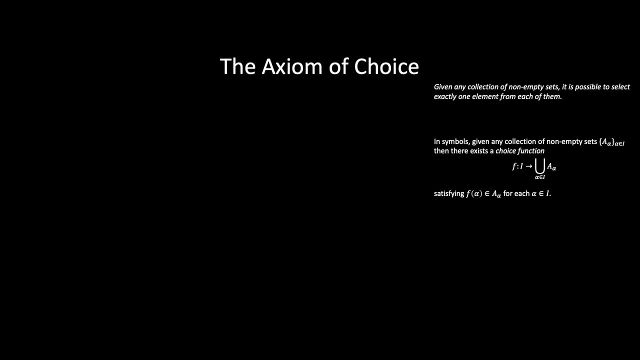 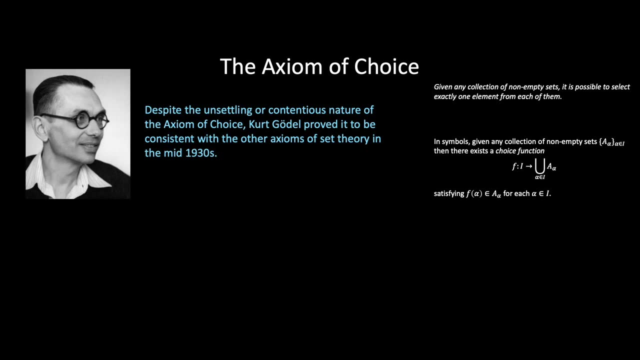 hand, the axiom of choice is intuitive and, on the other hand, we have to accept some really weird stuff if we believe it's true. So, despite the unsettling or contentious nature of the axiom of choice, Kurt Gödel proved it to be consistent with the other axioms. 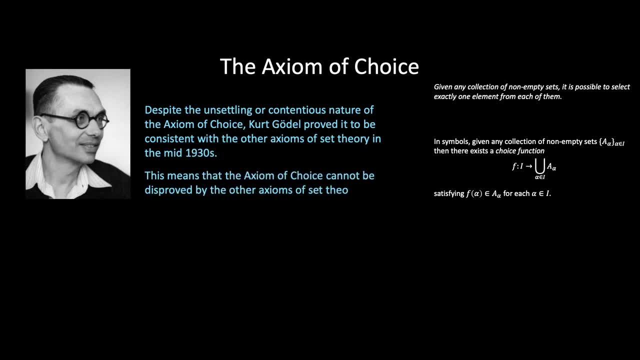 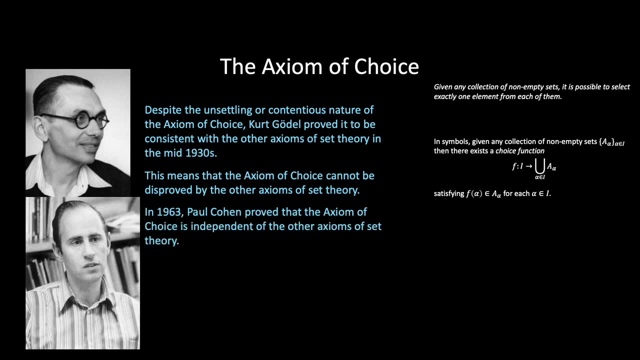 of set theory in the mid-1930s. That means that the axiom of choice cannot be disproved by the other axioms of set theory. In 1963, Paul Cohen proved that the axiom of choice is independent of the other axioms. 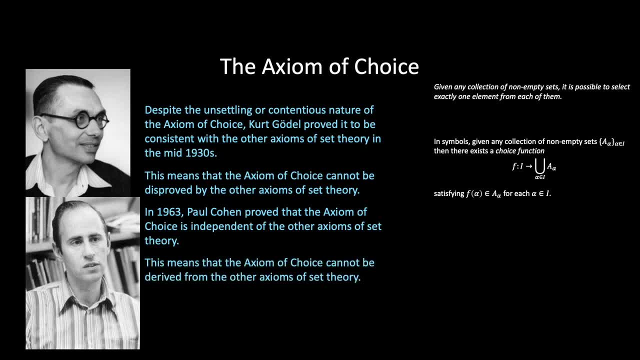 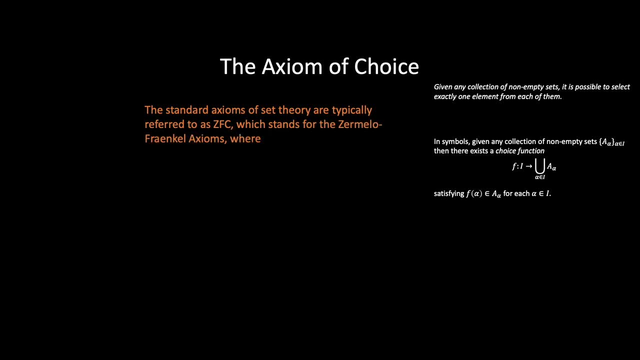 of set theory. That means that the axiom of choice cannot be derived from the other axioms of set theory either. The standard axioms of set theory that I've been referring to are typically referred to as ZFC, which stands for the Zermelo-Fraenkel axioms, and the C indicates that we are including. 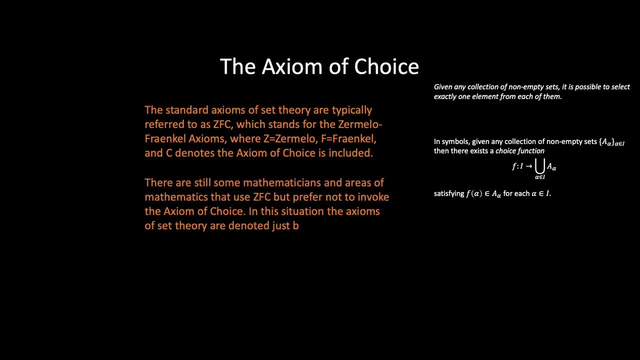 the axiom of choice. There are still some mathematicians in areas of mathematics that want to use the Zermelo-Fraenkel axioms but not the axiom of choice, and in that case those axioms are typically just denoted by ZF. 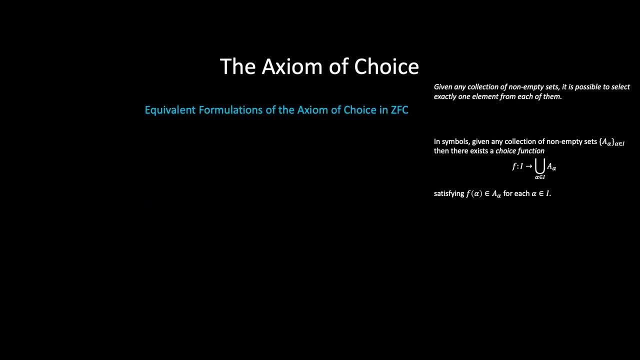 Now let's look at some equivalent formulations of the axiom of choice in ZFC. That means that if you believe the axiom of choice, then you also believe any one of these, and vice versa. So the well-ordering principle was proved by Zermelo in 1908.. It says that any set can 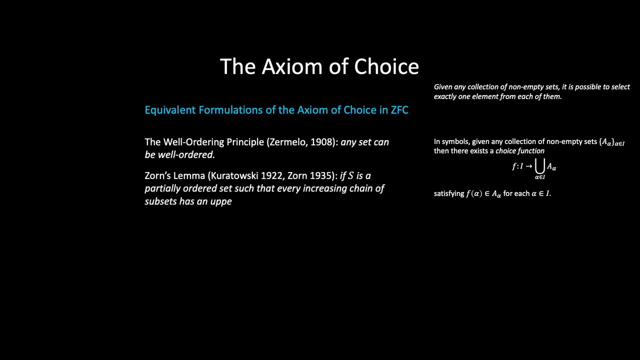 be well-ordered. Zorn's lemma says that if S is a partially ordered set such that every increasing chain of subsets has an upper bound, then S has a maximal element. Another equivalent result to the axiom of choice is that any family of non-empty sets 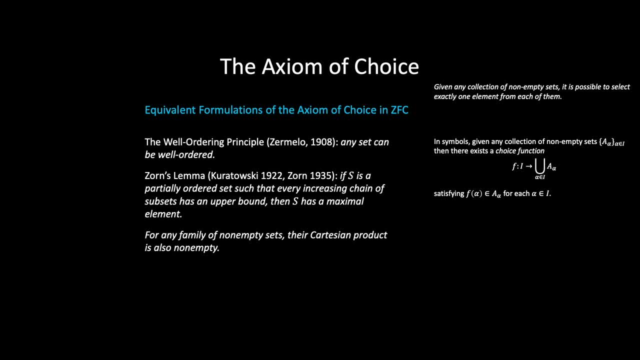 is such that their Cartesian product is also non-empty In topology. Tychonoff's theorem, which was proved to be equivalent to the axiom of choice by Kelly in 1950, says that the Cartesian product of a family of compact sets is always. 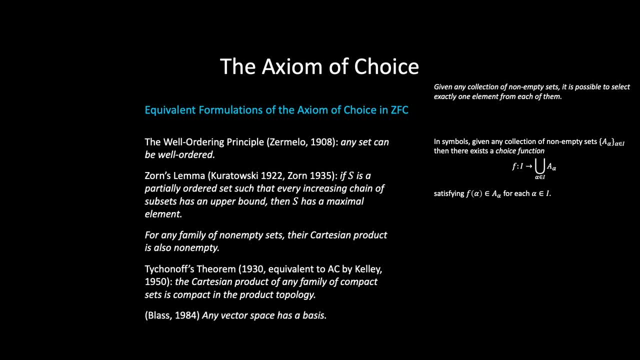 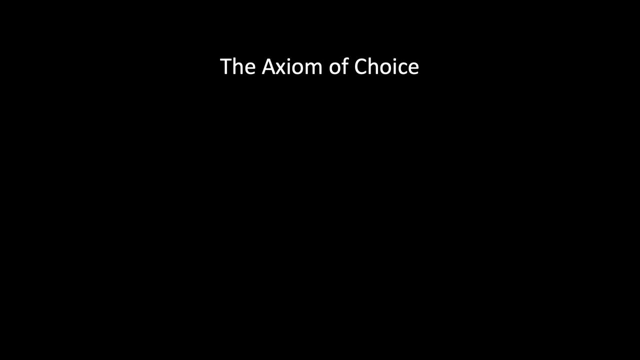 going to be compact in the product topology. And finally, Blas in 1984 proved that the axiom of choice is equivalent to assuming that any vector space has a maximum element. The last thing we'll do in this video is use the axiom of choice in a proof and we'll 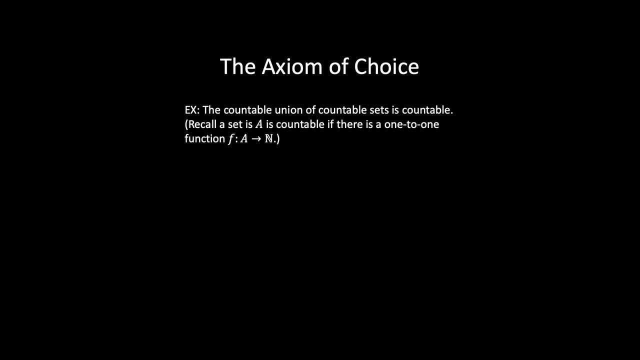 prove that the countable union of countable sets is countable. We'll call the sets countable if there is a 1-to-1, in other words injective function from the set to the natural numbers. So here's the proof. 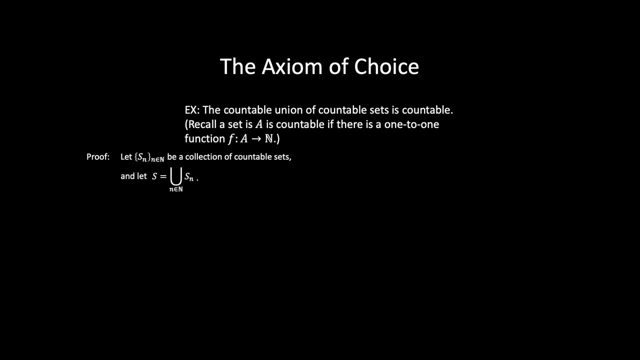 Let's let S sub n be a collection of countable sets and let's let S be the union of all of these. So for each natural number, we're going to let fancy F sub n denote the set of all 1-to-1. 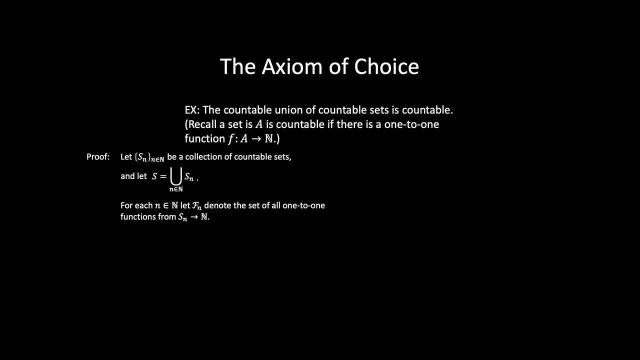 functions from Sn to the natural numbers, And we know that each of these F sub n's has an element. since each S sub n is countable By the axiom of choice, we can choose one function, little f sub n, from each of the. 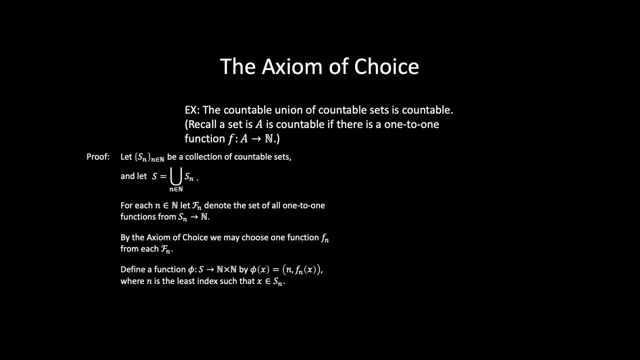 set's fancy F sub n. And what we'll do is we'll define a function phi from S to the product n cross n by phi of x is equal to the ordered pair n comma F sub n of x. Here n is the least index, such that x is an element of the set S sub n. 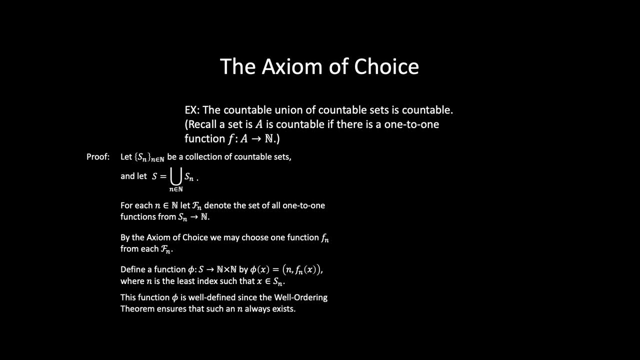 We know, since x is in the union of all the S's, it's in some S sub n. So since the natural numbers are well-ordered, it makes sense to go find the first n for which x is in S sub n. So that's why this phi is well-defined. 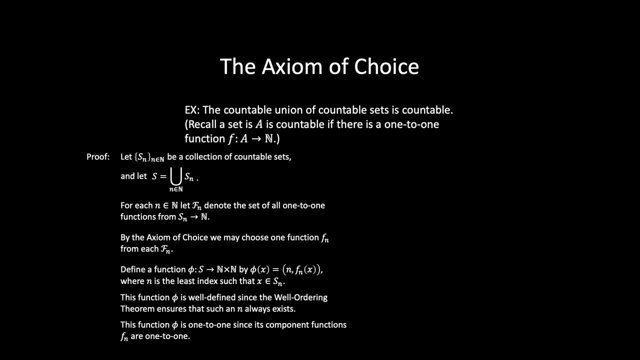 Now this function, phi, is 1-to-1, since its component functions, F sub n, are each 1-to-1.. Remember F sub n came from the set of all 1-to-1 functions on Sn to the natural numbers. Now, since n cross n is countable, there exists a 1-to-1 function, alpha, from n cross n to the.